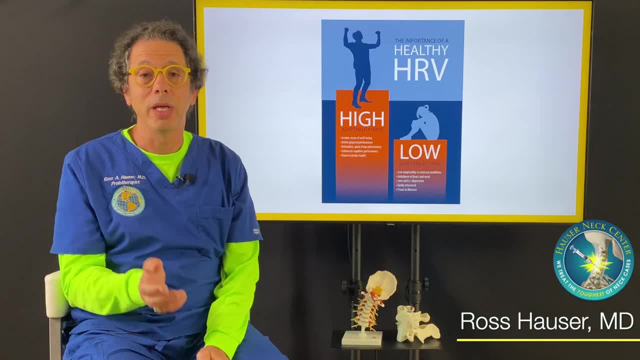 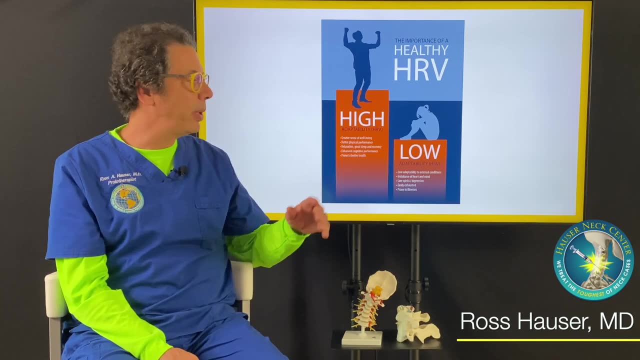 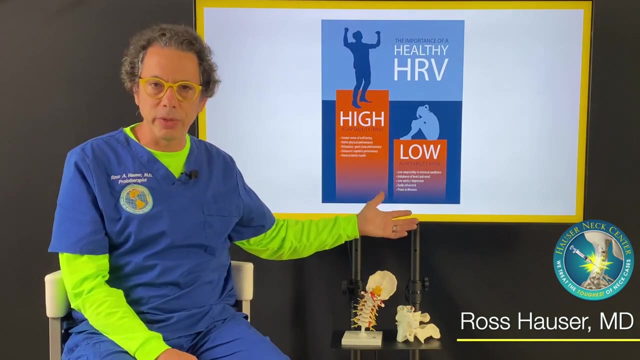 resistance to stress, and we all know right now you need to have a really high vagal tone to be healthy, To be vibrant, to be happy. When people have a low vagal tone, they can't handle stress so good. They're much more prone to getting illnesses, and these illnesses can occur all over the body. 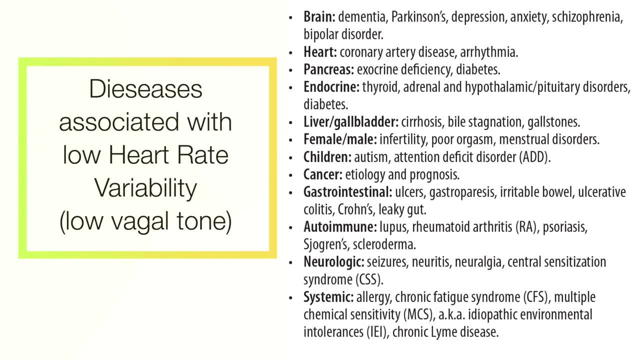 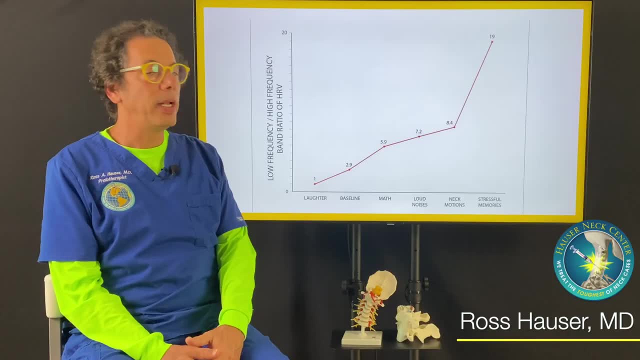 They tend to have depression or they might have other signs like brain fog or melancholy and other psychological conditions. They're easily fatigued and, of course, they're prone to illness. Now, this is an autonomic nervous system test that we did in the office in one individual, So what? 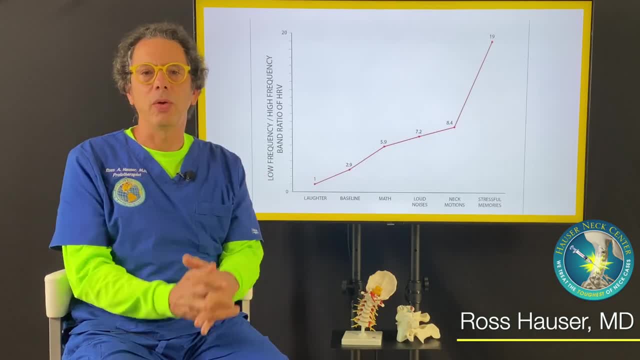 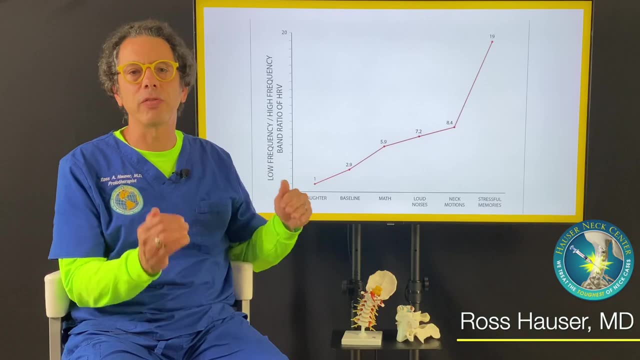 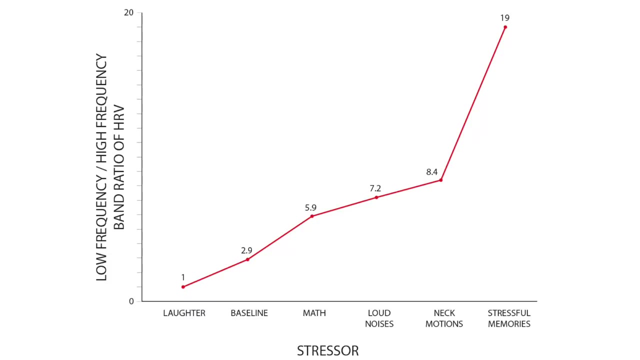 we do is we put electrodes on the person, like on their fingers, and what the probe is measuring is their heart rate variability and the various components of their heart rate variability. We can see that when the person had a stressful memory, just one stressful memory: the sympathetic. 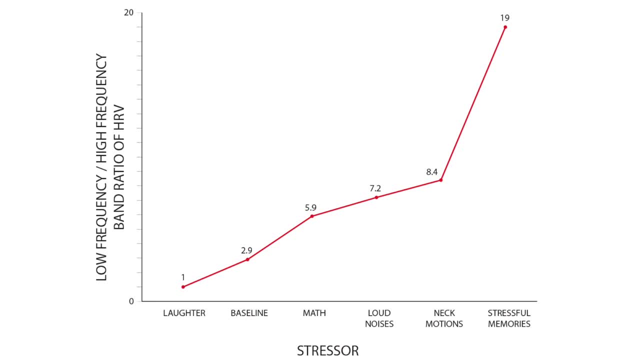 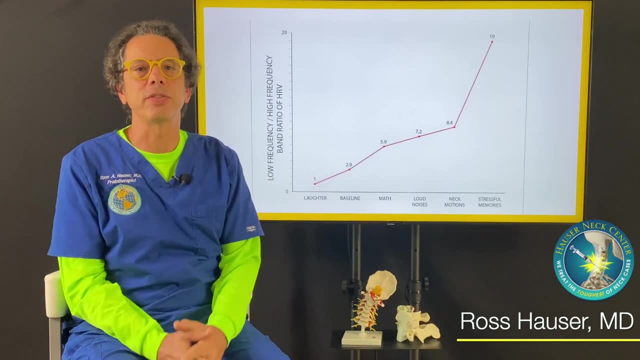 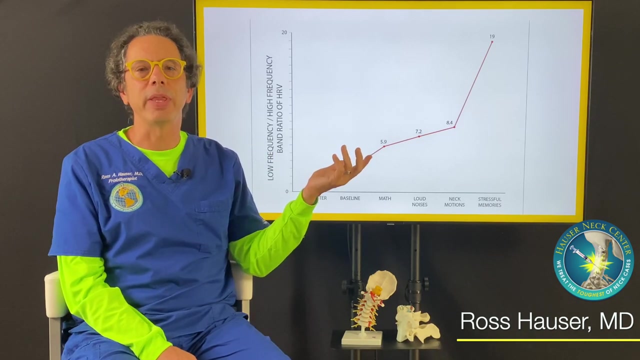 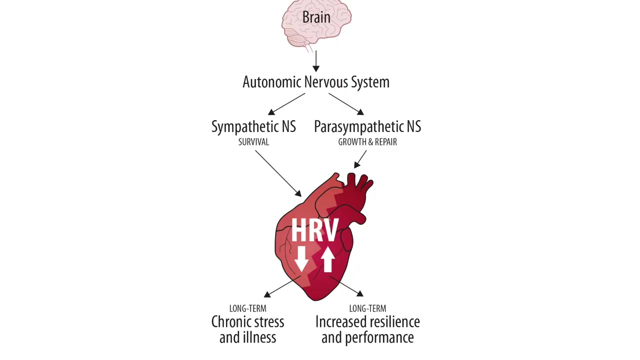 system went way, way up, basically 19 times the parasympathetic system. The sympathetic system is the stress system, So this person, just with one simple memory, became sympathetic, dominant, And then eventually, when we got the person to laugh, the sympathetic system and the parasympathetic 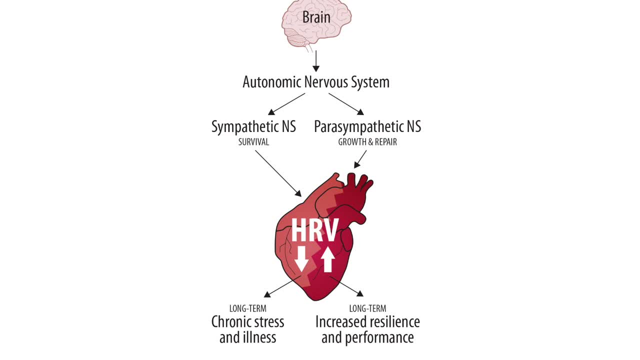 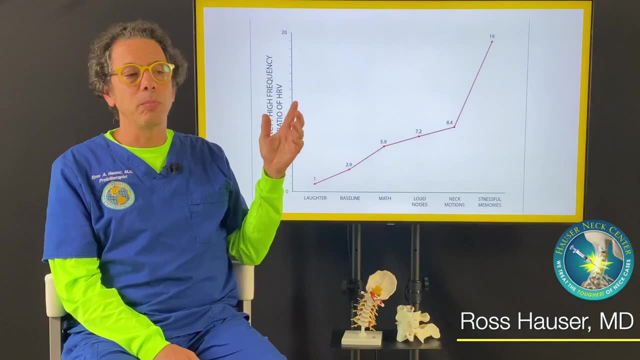 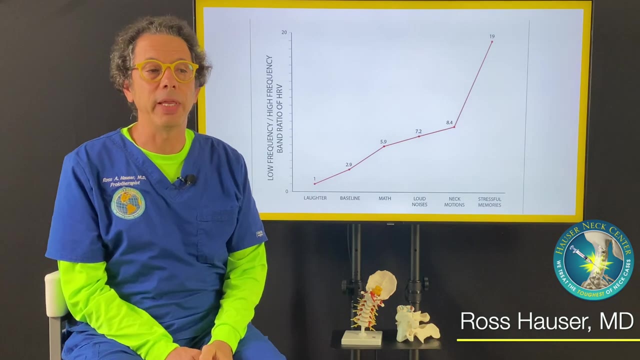 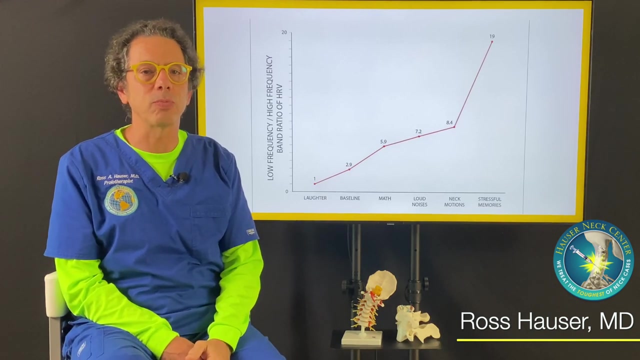 system was in balance. So heart rate variability testing can show us really how the person's doing as it relates to thoughts, memories, relationships. We can show the picture of somebody you know, just somebody that they might struggle with and just see what happens to their sympathetic system, their autonomic nervous system. just 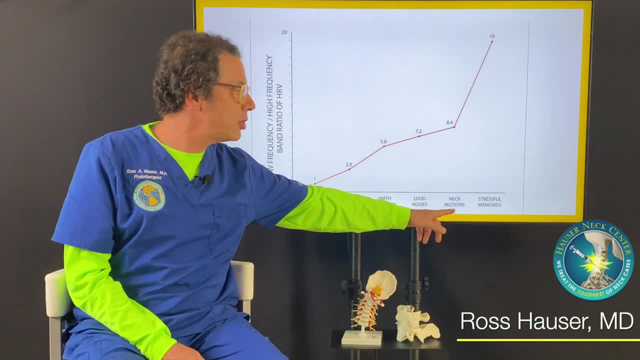 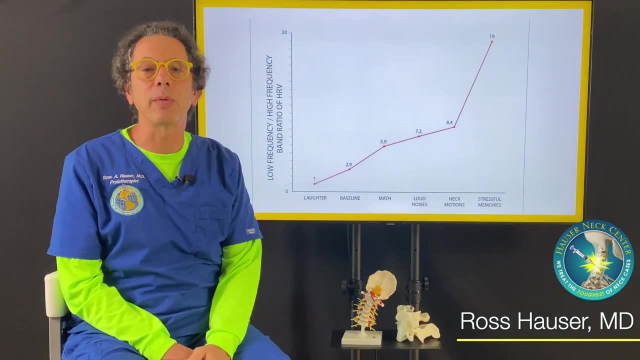 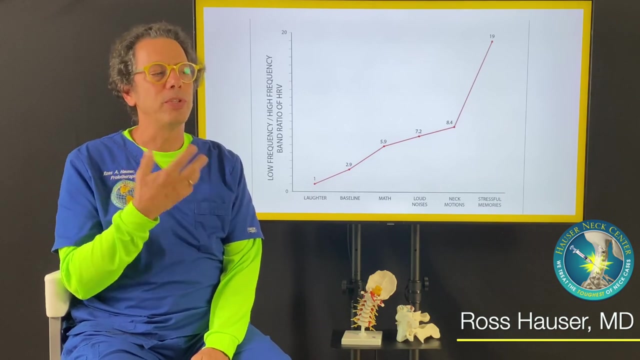 by that picture. We can also do neck motions. You could see the second most stressful event For this person beside the stressful memory was a certain neck motion, because there's definitely people that they can tell that when they move their neck in a certain position.